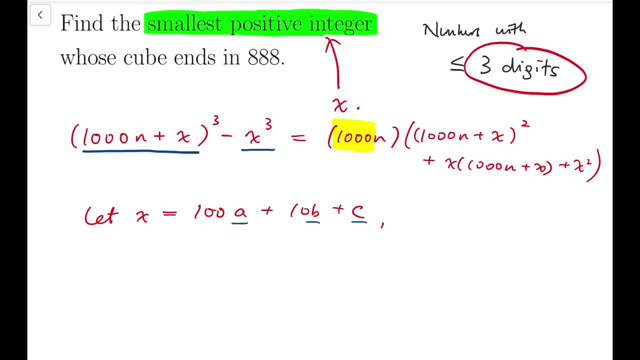 the digits of x- and I'm going to use notations in modular arithmetic, which is that x cubed is congruent to eight, eight, eight mod 1000. now from this we know that, in particular, x cubed is congruent to eight mod 10. now from this we can already deduce one of the 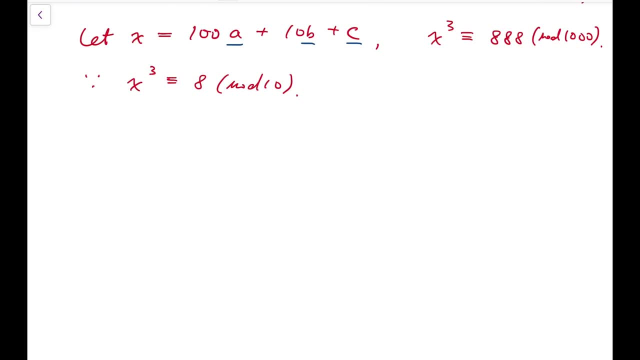 values of a, B, C. notice that for cubes, when I take mod 10, it can either be: 0 covers 0- we were 0- 1 cubed equals to 1, 2 cubed equals 8, and so on. 27, 64, 125, 216- I could i have the whole numbers- and then 2007, 40, free. 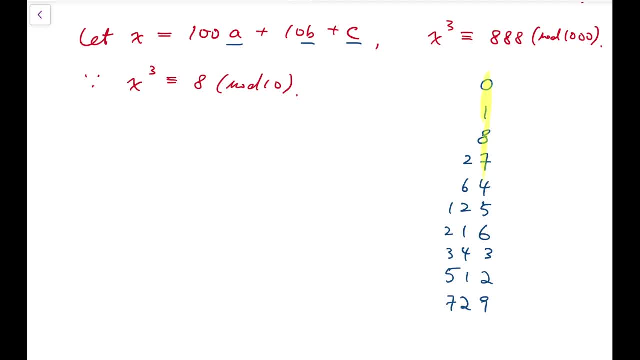 512, 729 and then the remainders repeat. now you have más 받, founding date. now we started off with a not Notice of system numbers. now, what we are going to Now, from this we know that we can only have a cube to be congruent to 8 mod 10 if the number itself is congruent to 2 mod 10.. 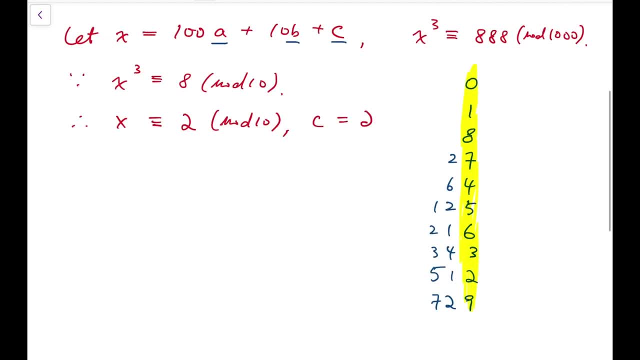 That means the last digit of x is 2.. So that means this c equals 2.. Now we can move on to solve the next digit, which is b. So from this result I can say that x is equal to 100a plus 10b plus 2.. 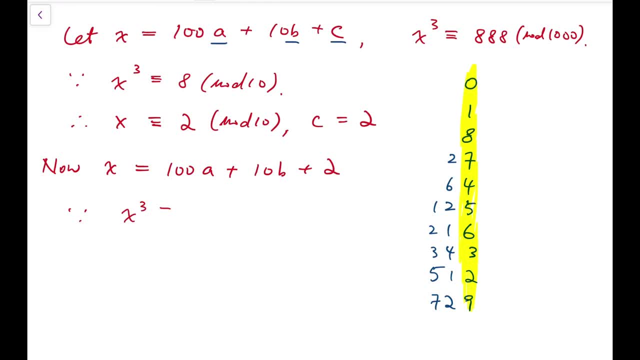 And I will consider mod 100 instead. Again from the same Condition, I can say that x cube is congruent to 88 mod 100.. And we know that x is congruent to 10b plus 2 mod 100.. 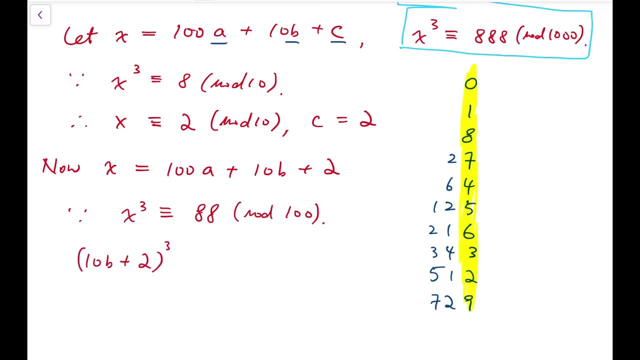 So I can simply expand 10b plus 2.. I can ignore the 100a term Now using the binomial theorem: 10,000b cubed plus 3 times 100b, squared times 2 plus 3 times 10b, times 4 plus 8, is congruent to 88 mod 100.. 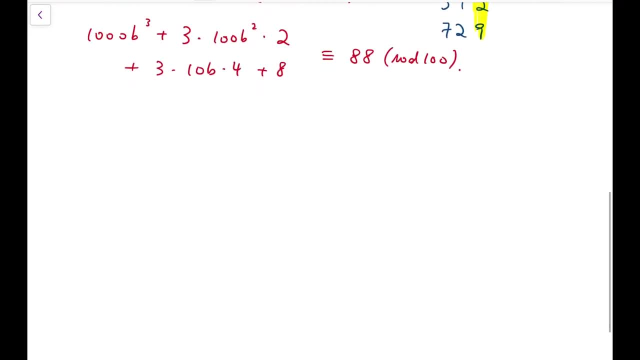 Now simplifying. we know that 120b is congruent to 80 mod 100.. So to simplify things, I'm going to rewrite this back into an equation, but not simply congruence and modular arithmetic. Let 120b to be equal to some multiple of 100b. 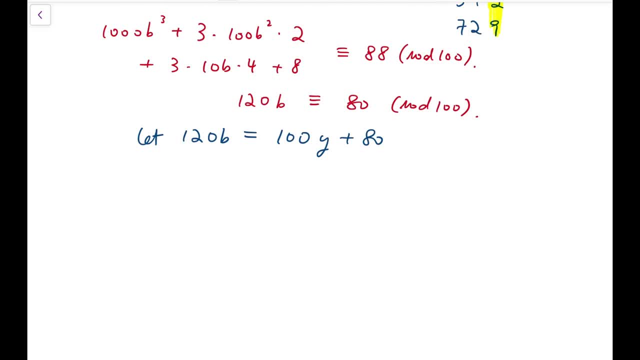 200 added by 80. Now we can divide both sides by 20. So that then 6b equals 5y added by 4.. So at the end I'm going to write b in mod 5. Biology course. 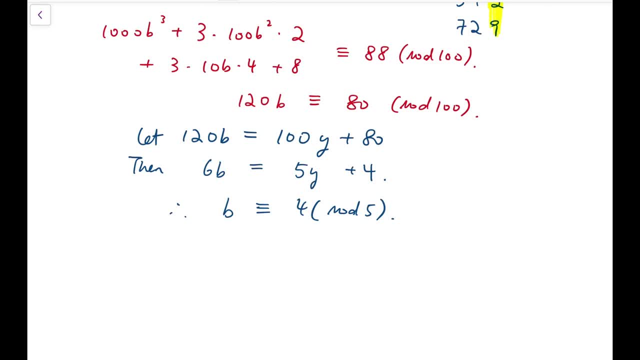 Thank you, See you soon, Bye, Bye, Bye, Bye. we know that I can only say multiples of b, to be some multiple of 5 and by 4, so at last I'm going to write b in terms of mod 5, now knowing that b is again a. 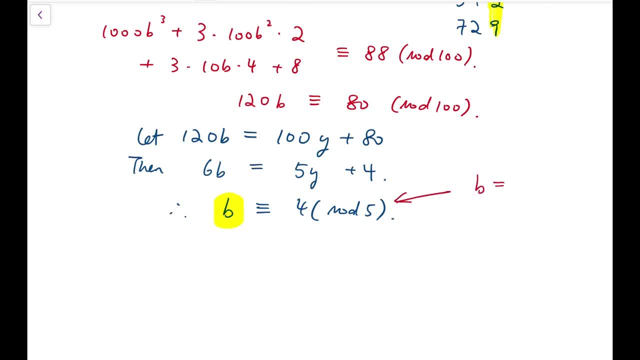 digit. it's a digit, so b can only be 4 or 9. now that means our last two digits of our answer X is either 42 or 92, but for both cases I can say that our answer X is congruent to 42 mod 50. we don't actually need to consider X mod. 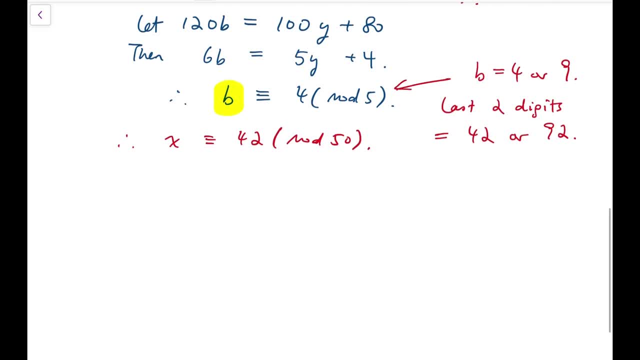 100, because mod 50 would be sufficient. the following steps are going to explain why this is the case. so for this I can rewrite the whole shape of X. I'm gonna say: let X equals 50n plus 42, and then I'm going to write X cubed in terms of N. 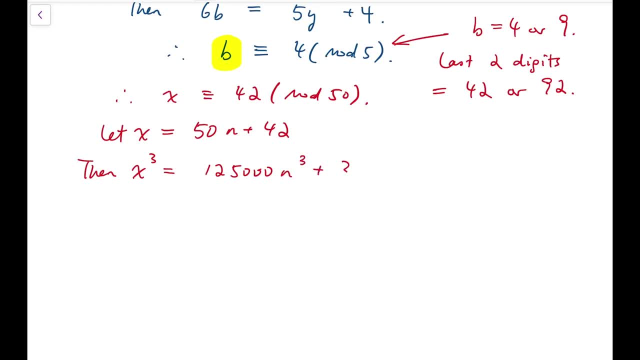 so the first term is 50n whole cubed. n whole cubed plus 3 times 2500 n squared, times 42, added by 3 times 50 n times 42 squared and at last added by 42 whole cubed. Now notice that 42 cubed is equal to 1764 multiplied by 42.. 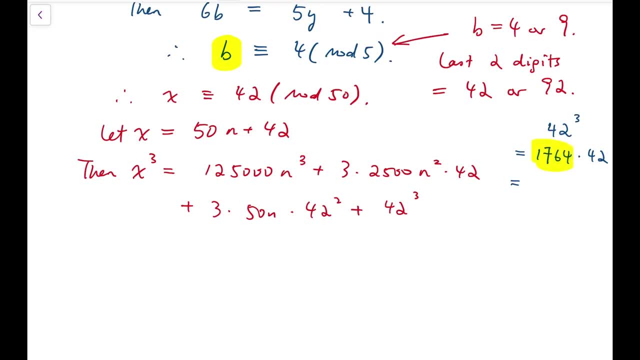 This is 42 squared, and so you will get at last 74,088.. Now back to x cubed. So this is congruent to only the last two terms. Let me explain this For the first term. it's clear that with the triple zeros this term is a multiple of 1000.. Now for the second term. 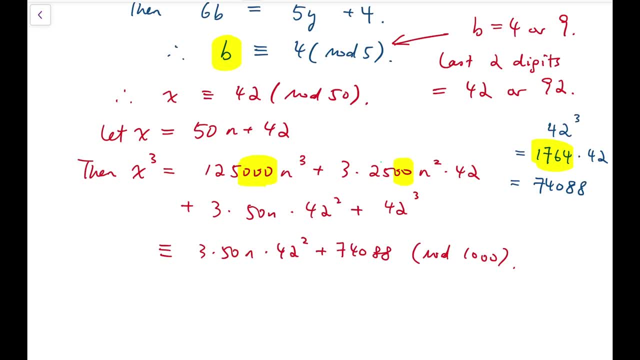 we already have two zeros and because 25 times 42 is a multiple of 10, so the second term will also become a multiple of 1000.. So that means I can completely ignore the first two terms, which makes our calculation much easier. 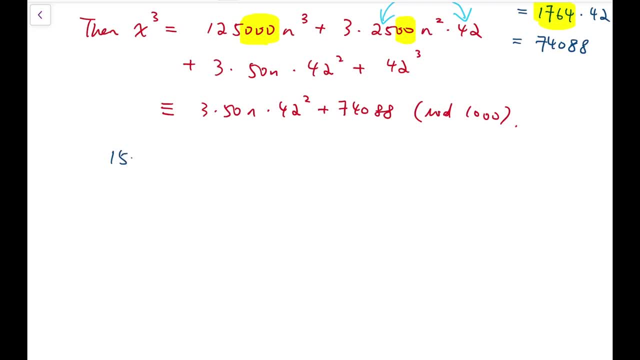 So from this we can say that 150 n multiplied by 1764 plus 74,088 is congruent to 888.. Now the second term is 106 mod 1000.. So, as you can see, the first two terms are equal to 106 mod 1000,. 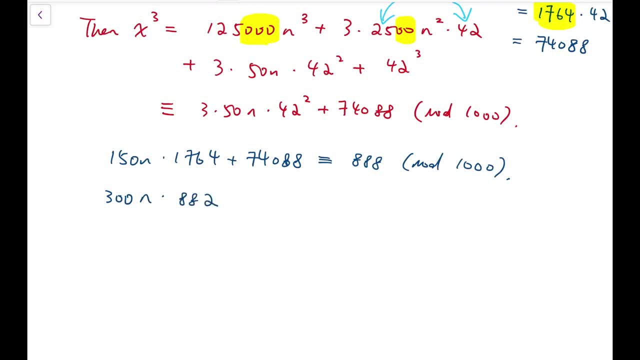 as required by the problem, And again I'm going to simplify that a bit. I'm going to rearrange the factors in the first term. As you can see, I doubled 150, the other number. The purpose of doing this is to show that this term is. 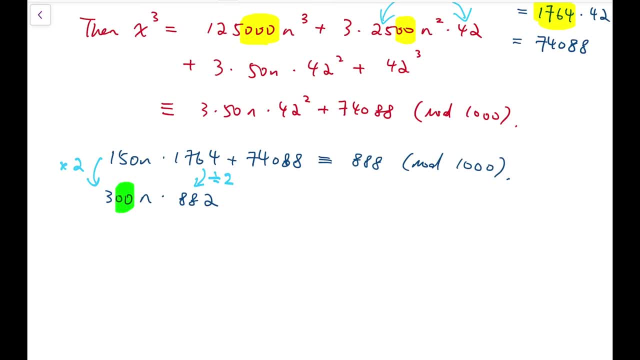 actually a multiple of a thousand from the double zeros, and this term is congruent to minus 73200 mod 1000. and then again I'm going to rewrite that back into an equation. rather than just congruence in multiple arithmetic, I'm gonna let this be some multiple of. 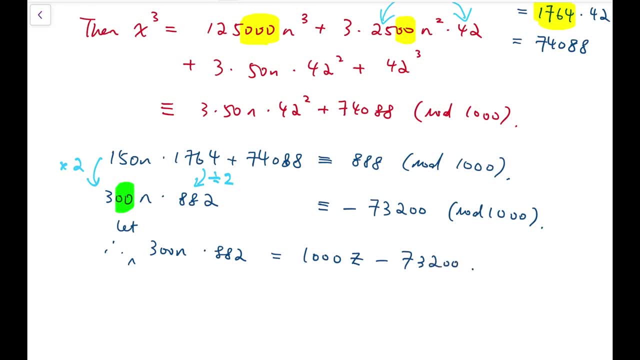 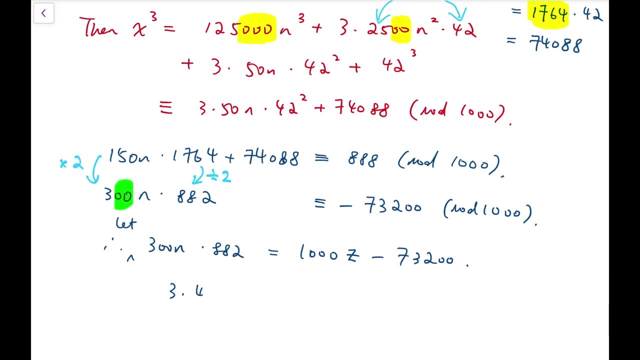 1,000, subtracted by 73,200.. I'm going to divide both sides by 200, so it gives 3 times 441, taking away these two zeros and dividing this number by 2, and that I will get division by 200. 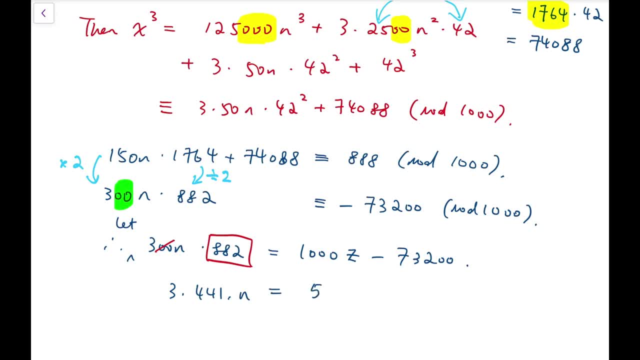 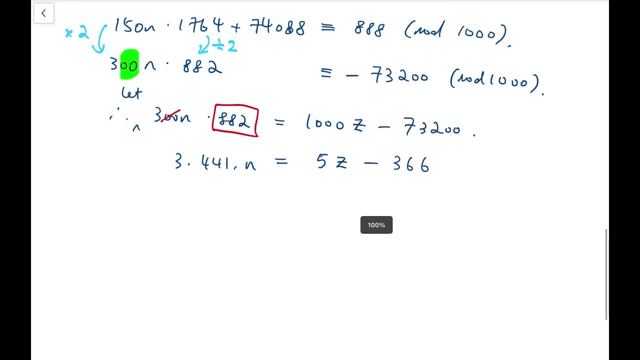 so that's 3 times 441 times n equals 5z minus 366. and now, using a similar argument as above, we know that we are going to rewrite n in terms of mod 5, so I'm going to take mod 5 on both sides and I get 3n. 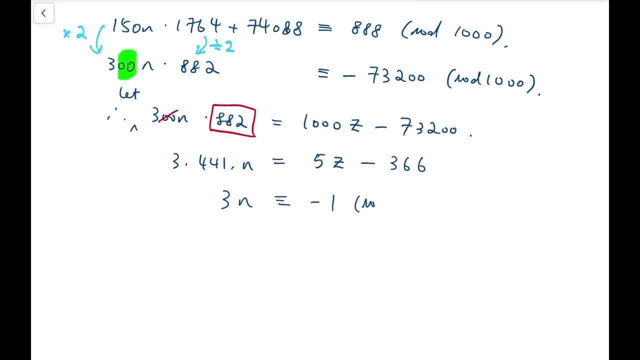 is congruent to minus 1 mod 5, and we know this is actually equivalent to 4 mod 5 and by checking you know that n can only be 3 mod 5. now, combining all the results, we know that x is equal to 3 mod 5, so we know that x is equal to 3 mod 5.